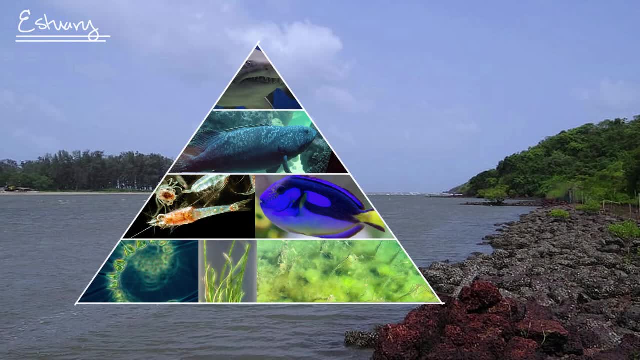 for, let's say, this estuary that we're looking at right over here, it might look something like this where, at the bottom layer, these are the primary producers, And we've studied this in other videos: Primary producers In a marine environment. 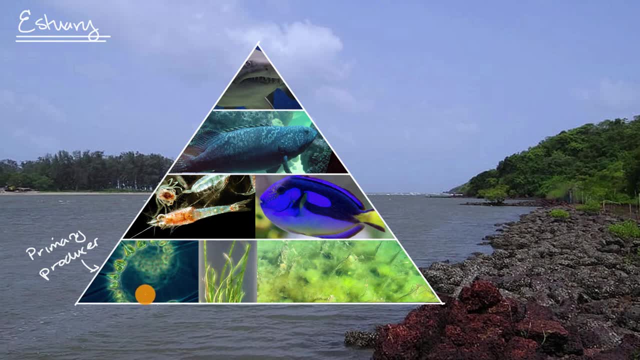 these would be things like phytoplankton, Phyto. they're doing photosynthesis and they're plankton- Plankton is a general term that comes from the Greek for drifter. This right over here is seagrass- also something that can photosynthesize. 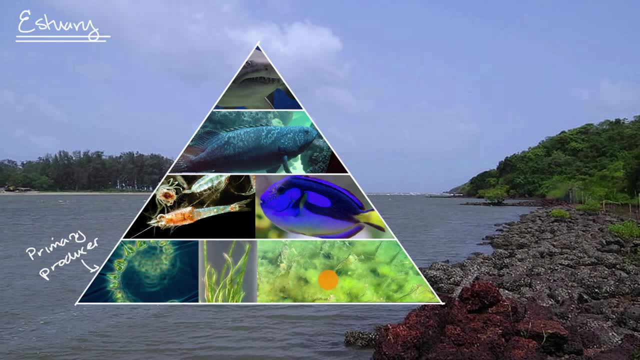 And this right over here is algae which I'm sure you have seen when you've gone to the sea or you've gone to a pond of some sort. And when we think of photosynthesis we often talk about terrestrial things, things like trees. 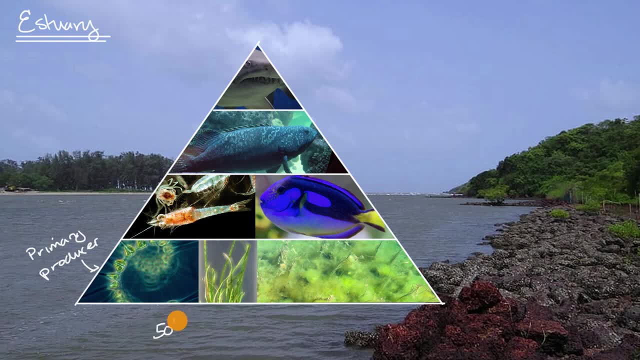 but a lot of us don't realize that 50%- that's a big number of Earth's photosynthesis, or net primary production, or organic energy compounds, is produced by floating photosynthesizers like phytoplankton and ultraplankton. 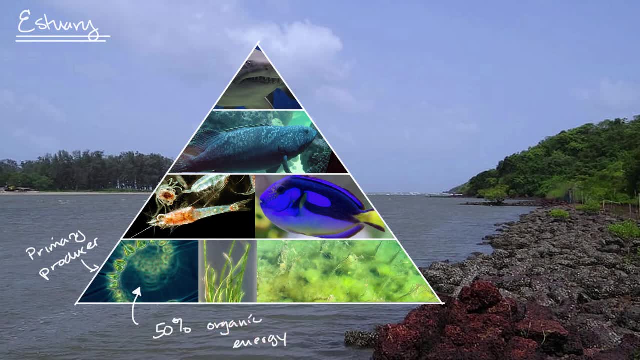 So things like this, things that you oftentimes don't see, And, as I mentioned, estuaries, tend to be quite productive. They actually are comparable to things like rainforests. Now, for the sake of making things tangible, this being an estuary which is very productive, 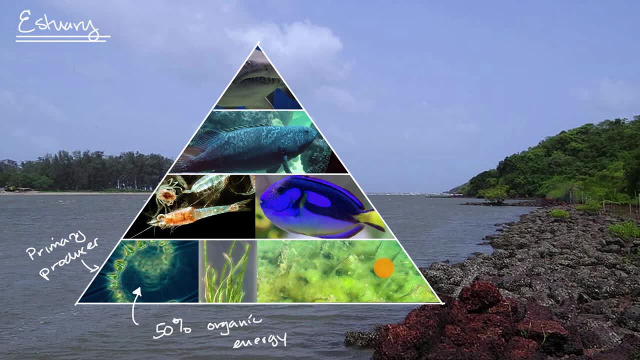 let's imagine that the net primary production from this first layer- we could think about it in terms of biomass- maybe it's about 2,000 grams per square meter per year, or we could think about it in terms of calories- This would be approximately equal to. 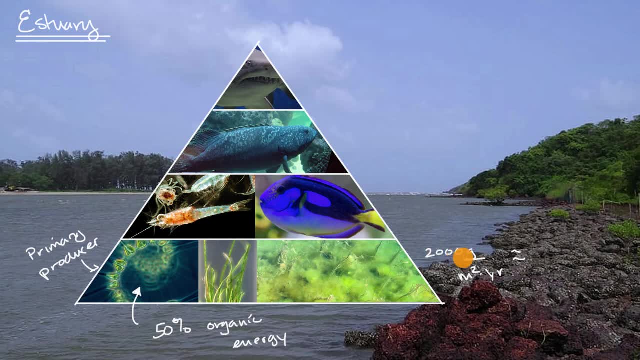 it depends on the type of biomass you're talking about, but you have roughly four kilocalories per gram, So that would be roughly 8,000 kilocalories per square meter per year. That's the net primary production of this first layer of the primary producers. 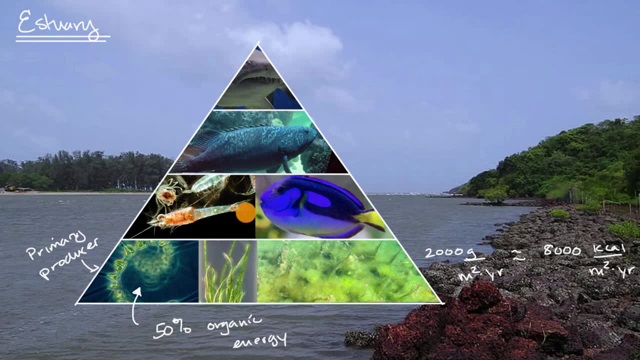 Then what would we see at the next layer? Well, we know that not all of that energy can be used by that next layer, which would be the primary consumers, And there's some examples here, and it's much more complex than what this pyramid depicts. 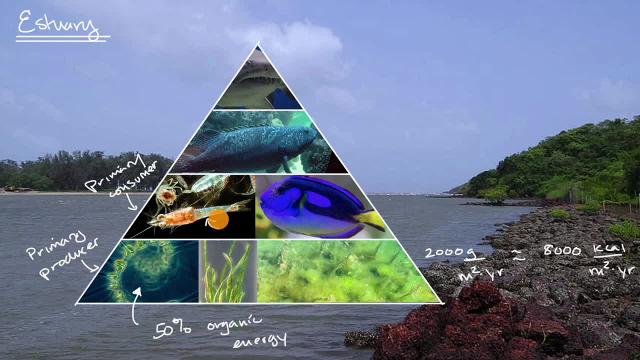 but what we see here, these are zooplankton, which are really- you could view it as- animal plankton. It's a large category of things. They have the word plankton in it, so they kind of have to go with the flow. 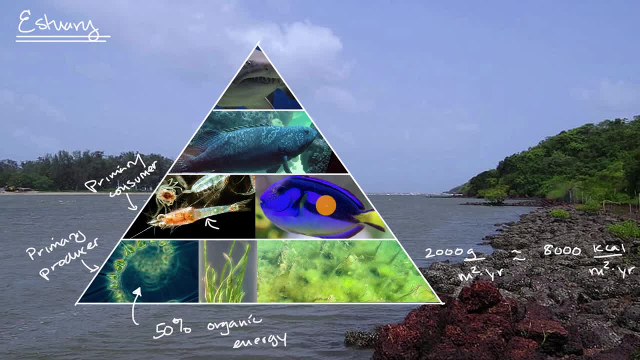 of whatever the tide is doing, whatever the current is, whatever the currents are doing. Another primary consumer could be a fish like this royal blue tang that might be eating plankton And the net energy that's available to the layer above. that is gonna be a small fraction. 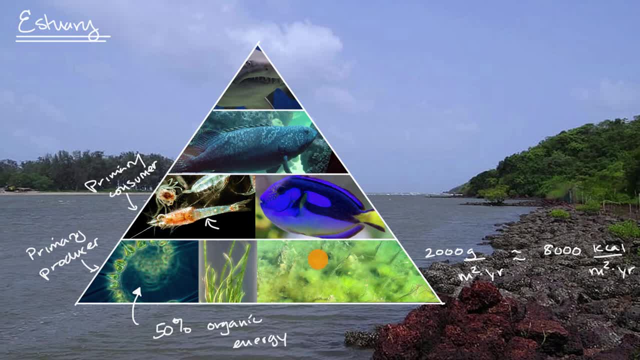 of the net primary productivity of that first layer. Typically it's about 10%. So there might be, instead of 8,000 kilocalories, 10% of that. we'd be talking about approximately 800 potential kilocalories per square meter per year. 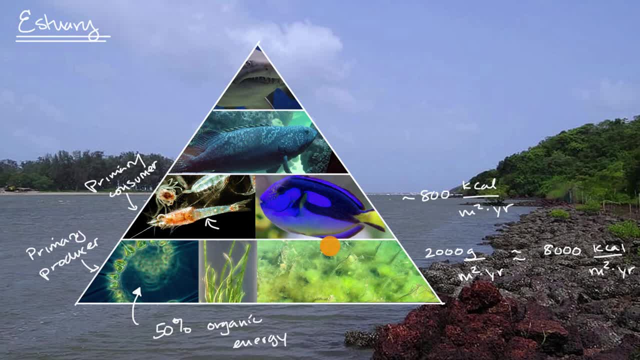 that would be available for the next layer. Now you might be saying, hey, where are all the other calories going? Well, remember, even in this first layer we said: this is net primary production. The growth would be even higher. 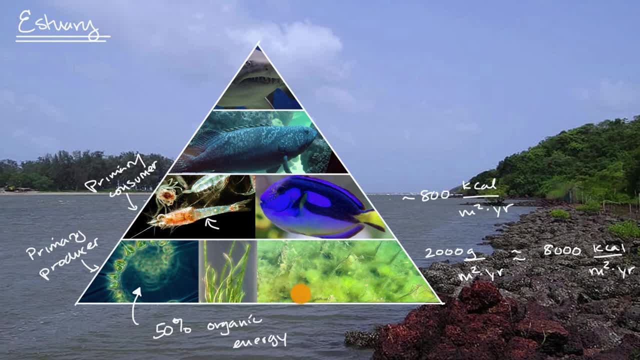 These photosynthesizers had to use that energy for things like respiration And even on the net basis. the reason why so much gets lost when you go to the next layer is these animals here. they have to use that energy to live. 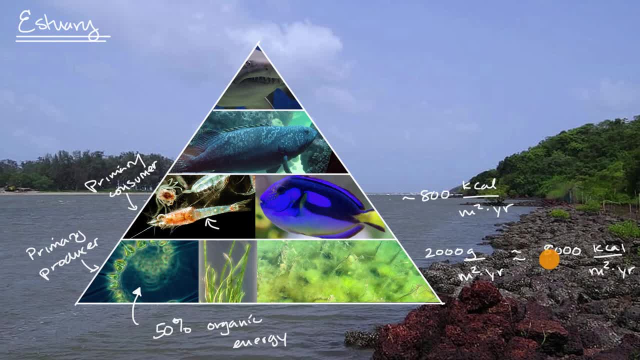 to do things like respiration And a lot of the energy that's available to them. a lot of this energy is just not consumable by the next layer, So it can become detritus, which is- you can just think of this- biomass. 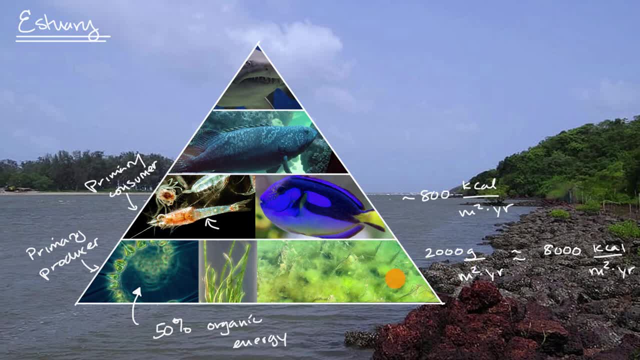 that is just laying around. Energy at every level can be lost to heat, can be used for movement, for growth. So you can imagine you get to a level above that We could call this secondary consumer. And this is just a picture of a grouper. 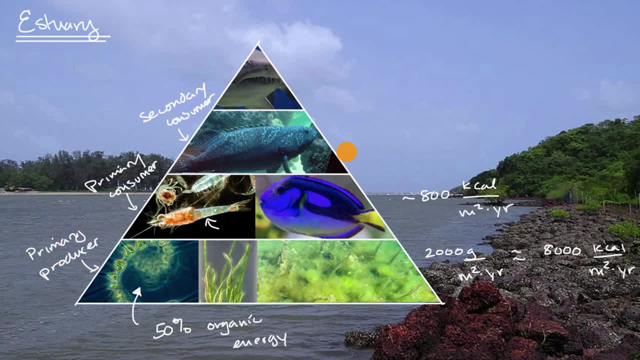 Marine ecosystems would be much more complex than this. But the net calories after the groupers live their life, et cetera, et cetera, that is available to the level above that would be roughly again 10%, So maybe 80 kilocalories per square meter per year. 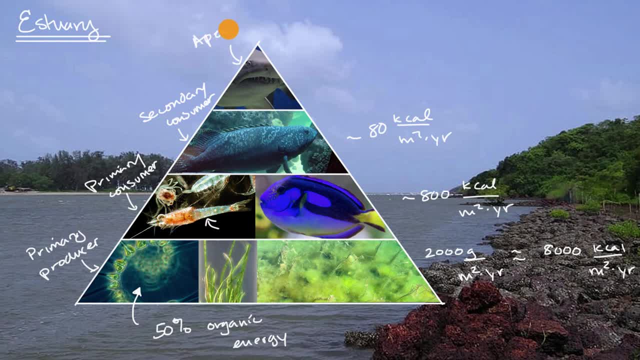 And then, at least in this example, at the top of this pyramid we have an apex predator, that is, a shark. What is available after the shark's done all of its business is roughly 10% of that, So approximately eight kilocalories per square meter per.